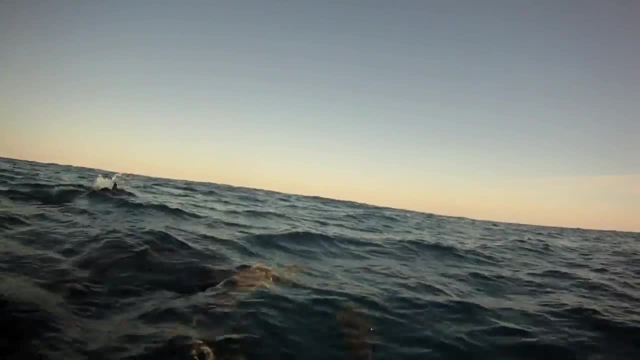 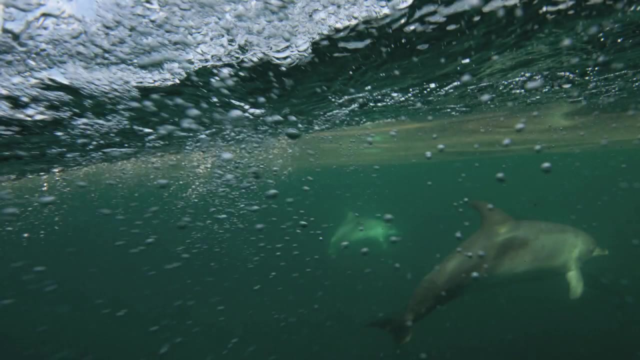 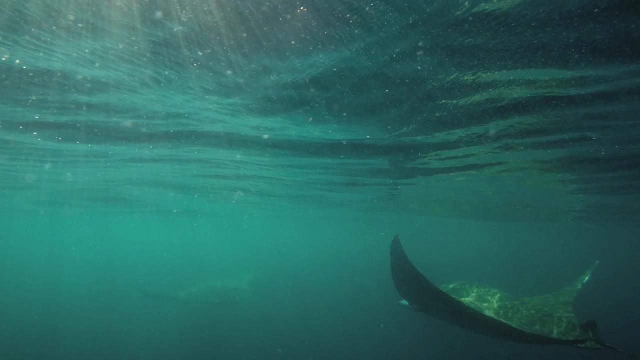 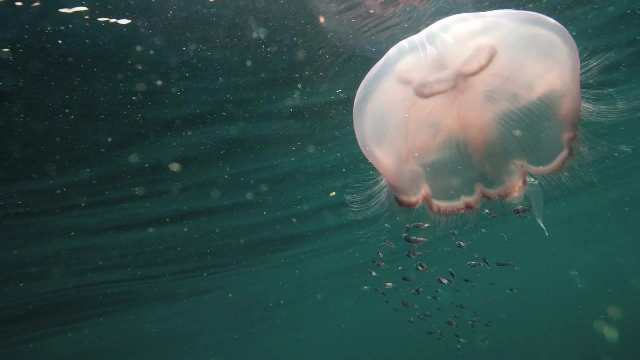 I come out to the shelf break at least once or twice a year and it was amazing to see the diversity of marine life down here. It was a great feeling to be trying to identify and understand how these creatures use their ocean environment and to use our understanding. 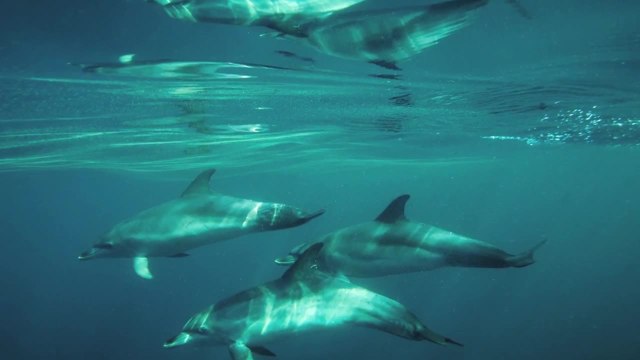 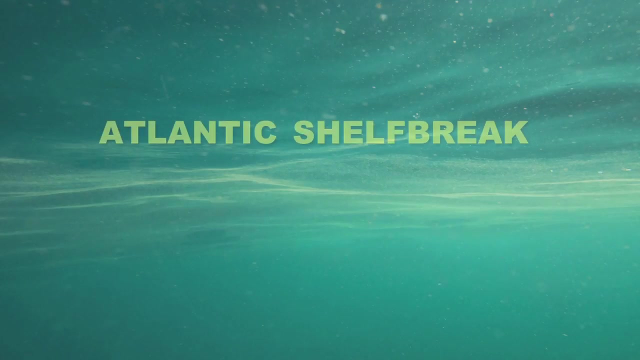 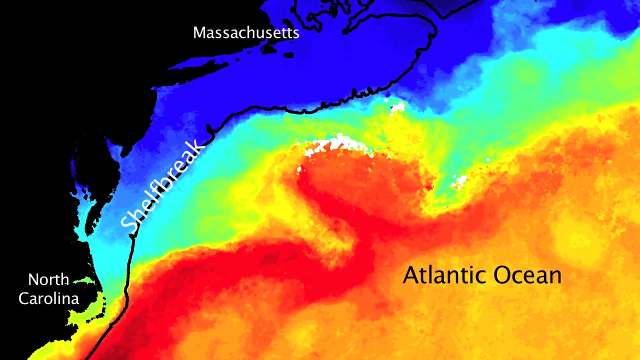 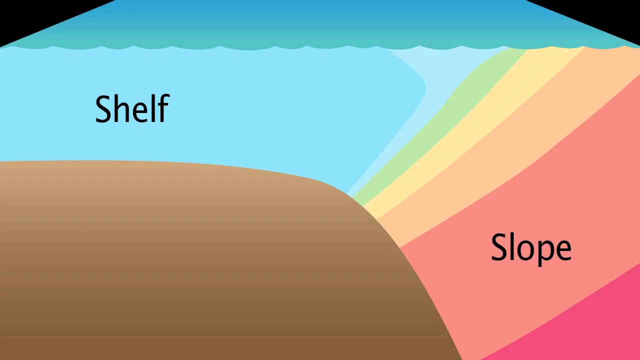 of the physical oceanography to try and imagine what these creatures' lives are like, to imagine how they go after their prey. The shelf break is the boundary between waters of the continental shelf and the deeper continental slope. The reason the shelf break is so important is that there's a persistent upwelling cell. 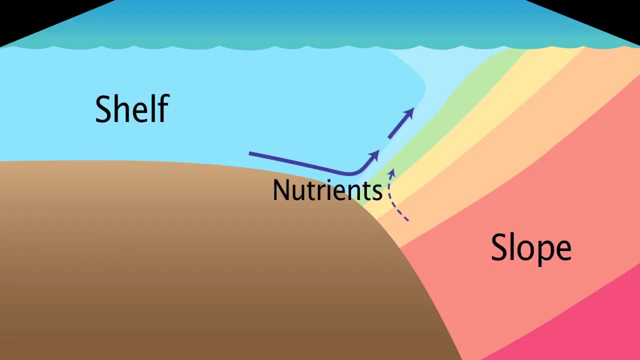 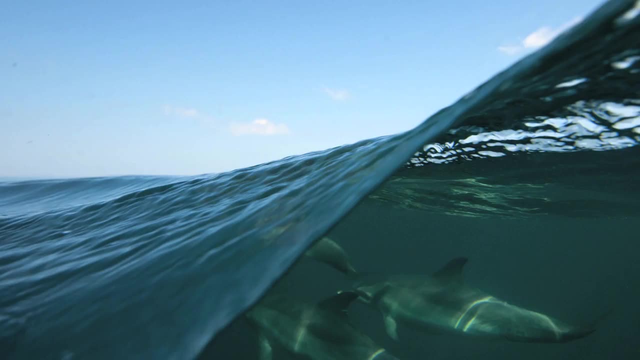 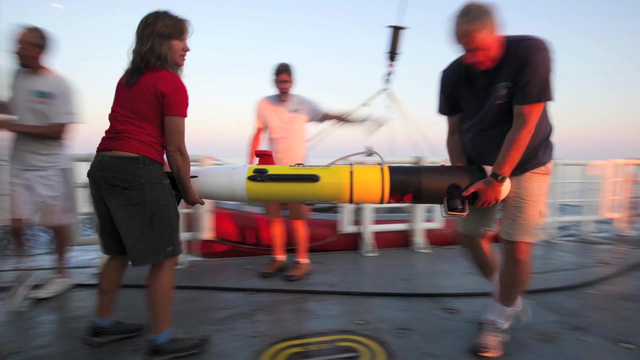 that tends to bring nutrients from deeper down in the water column, where the ocean is, where they're abundant, up into the near surface region where there's plenty of light. We think that marine life is abundant at the shelf break because of this upwelling cell. 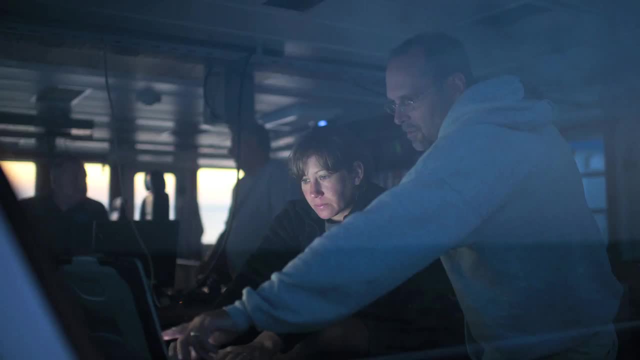 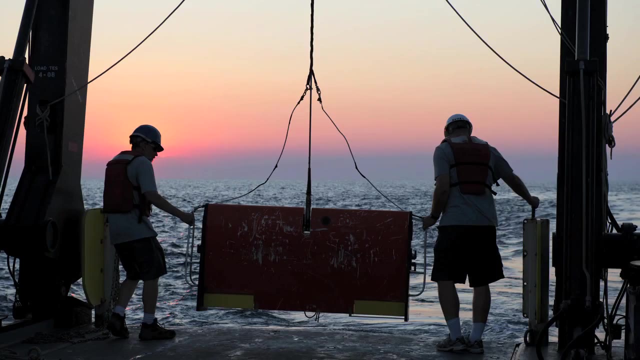 We're using two major tools for the physical oceanographic part of this project. During the night we do large, broad scale surveys with a toad undulating vehicle called a scanfish, and then during the day, we're going back to the shelf break and we're going back to the 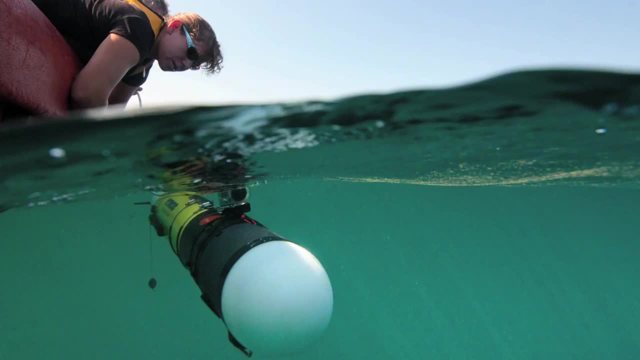 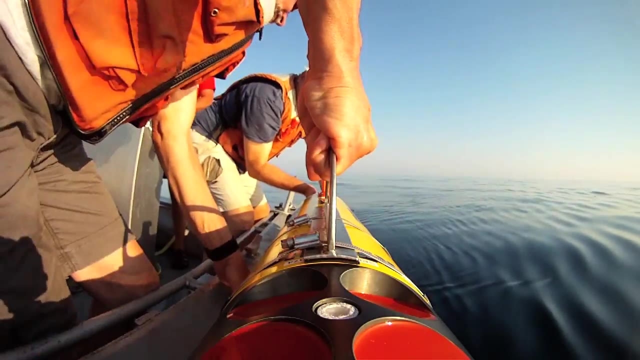 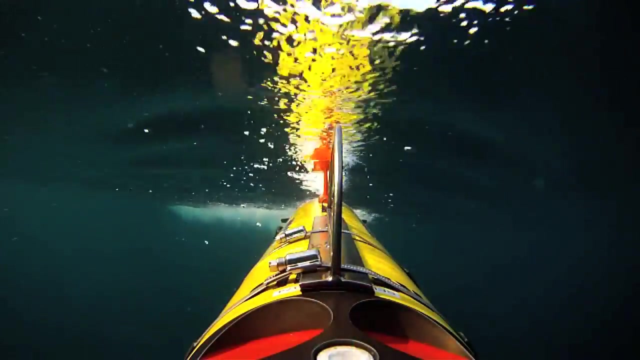 back and sampling it with an autonomous underwater vehicle, And that vehicle contains instruments for water temperature, the water salinity, but it also contains a very high resolution side scan sonar. Normally that's used to image the bottom of the ocean, but we're examining. 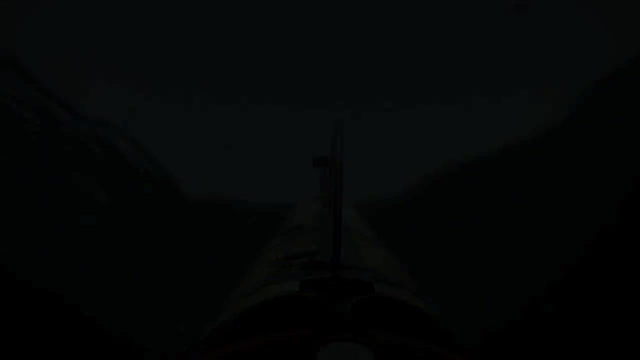 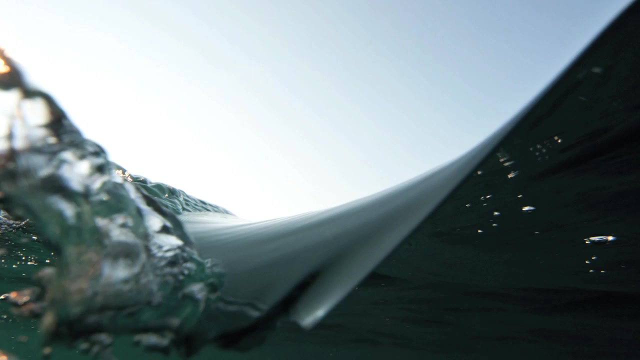 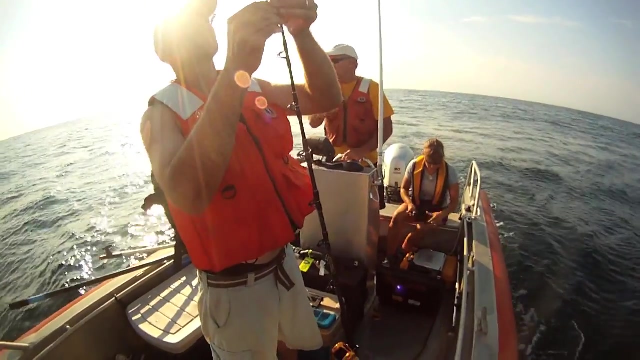 how well it can image fish schools. Oceanographers at any time can go out and find water. They never miss, And if they do, they probably shouldn't be oceanographers. The biology is difficult because of the unpredictability of it. You can't always go out and find fish or find the fish that 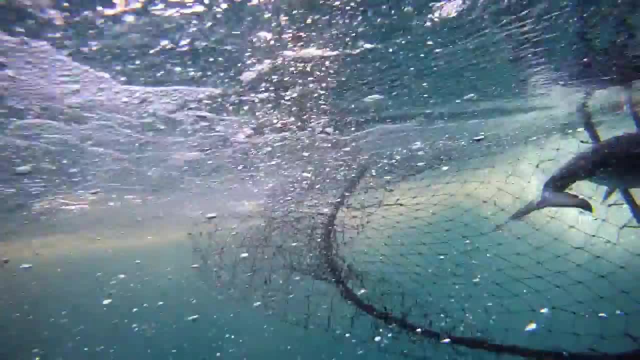 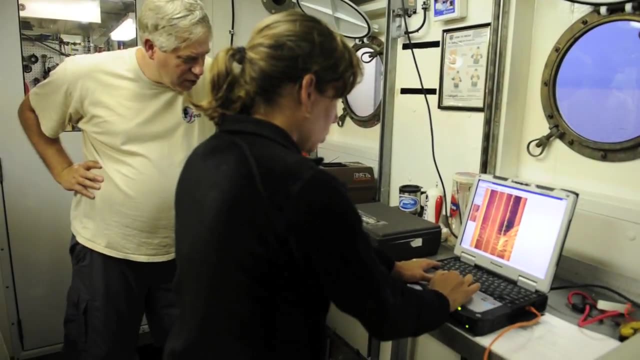 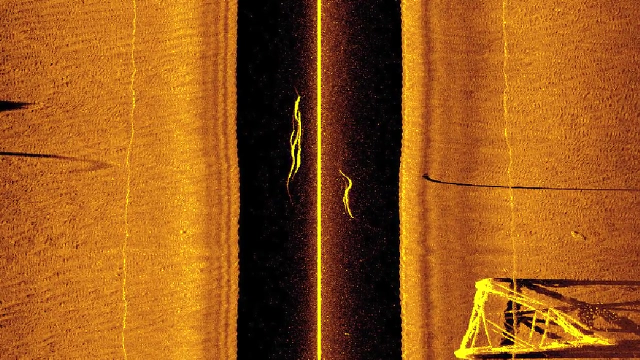 you want. You really never know where you're going to find them or what they're going to be doing. One of the most challenging things is identifying and calibrating the particular sonar return of the fish. You can't always know the type of fish it is because their different structure can reflect.